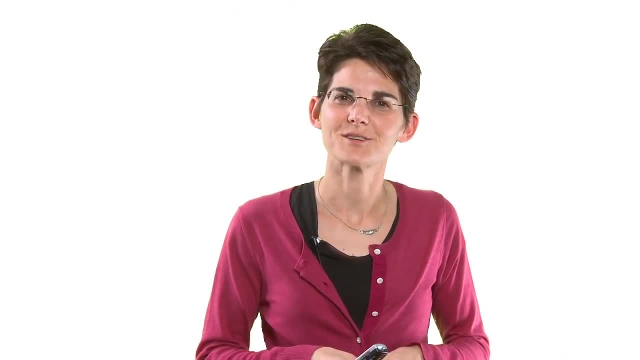 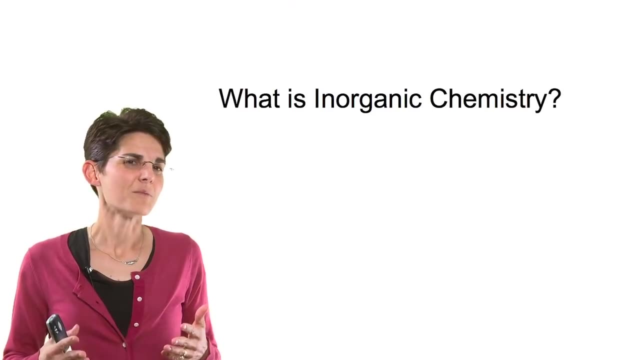 Hello, my name is Kathy Franz. I'm a professor of chemistry at Duke University, and today we'll talk a little bit about inorganic chemistry. So what is inorganic chemistry? You could probably come up with a lot of answers to that question, So let's focus on just a literal meaning One. it's: 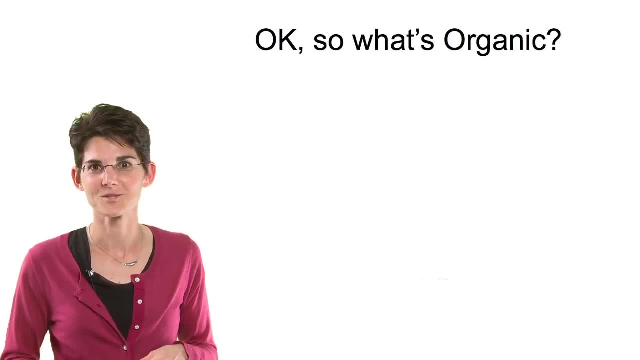 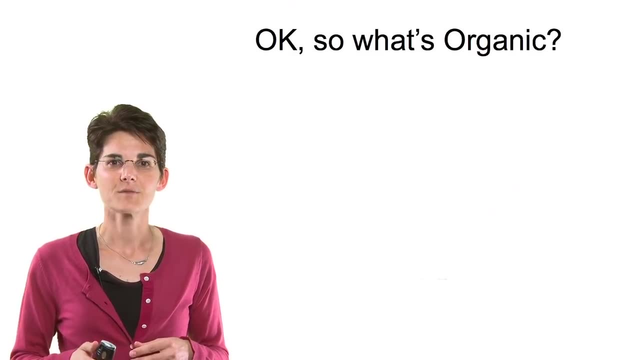 not organic. So that begs the question: what's organic chemistry? And here we can really take again a literal meaning and maybe a more chemical meaning. So if we take it literally from its word, we can say it's not, it's from an organism, So it's a living thing. Or, if we want to, 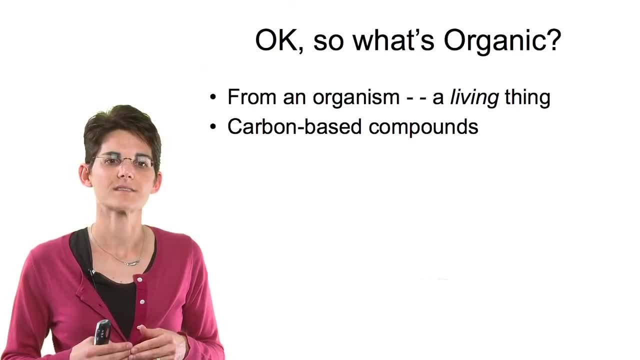 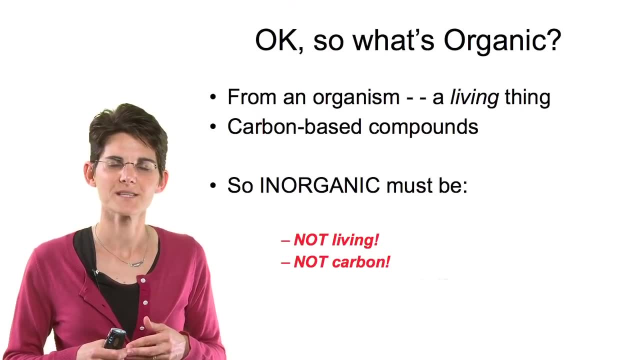 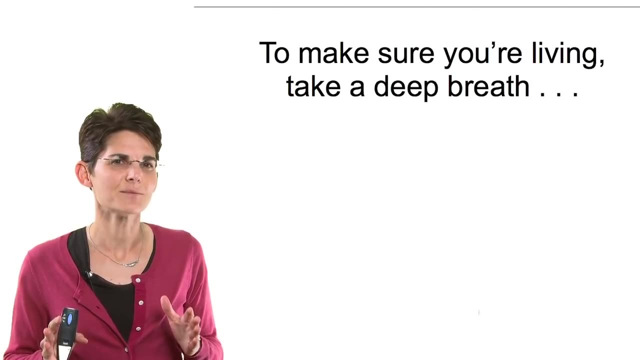 take a chemistry definition. we'll say organic chemistry's are carbon-based compounds. Okay, so then we're left with the definition for inorganic chemistry that it must be not living and not carbon. Okay, so just to make sure that you're breathing, take a deep breath. 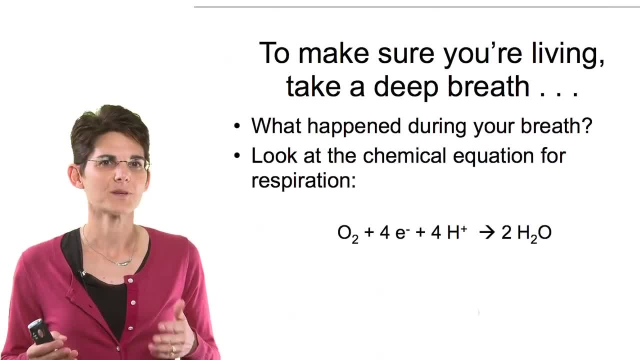 What happened in that breath? Again, a couple of things happened. You breathed quite a lot of things within the right phase of your organization. You breathed very little, Alright. so look, do you see that difference? Yes, in mostly nitrogen, but some oxygen also. and what happens to that oxygen? well, 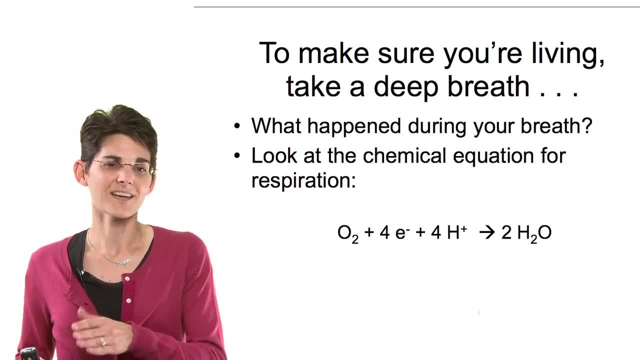 there's a lot of inorganic chemistry involved in that, but at the very end of the day that oxygen has to be reduced all the way to water and it takes our electron. it takes like four electrons that come really from the food you eat and turn and that goes into water. so here's our reaction: oxygen, o2 four. 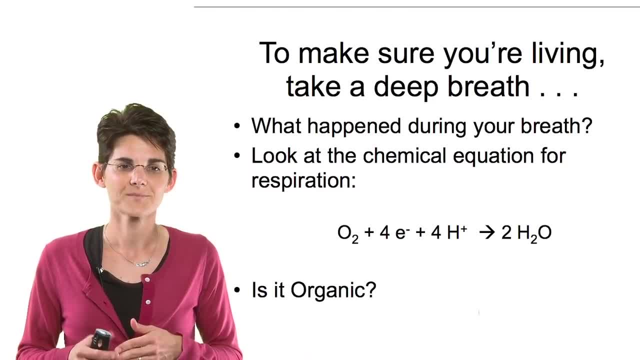 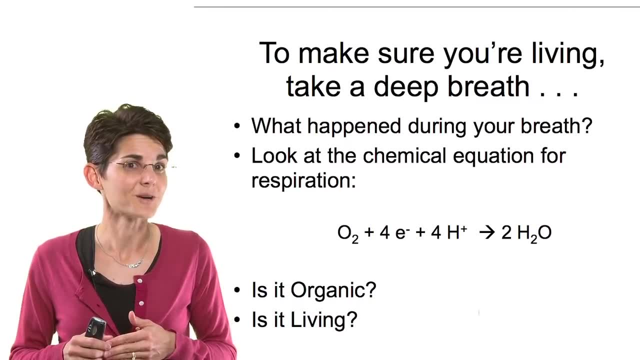 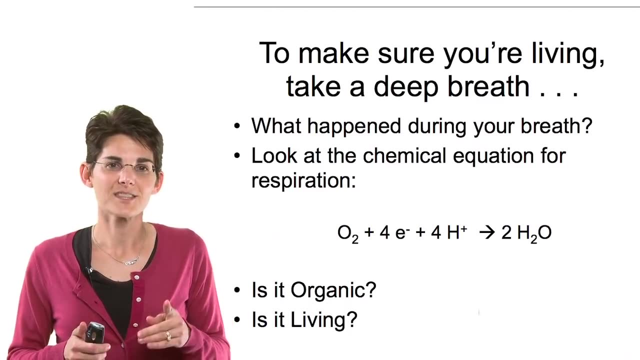 electrons, four protons, and we get two molecules of water. a couple of questions: is it organic? is it living? so now we have one of the world's most important reactions and it's not organic, but it is living, and this is inorganic chemistry. now let's take another look at this reaction in terms of where it happens. so 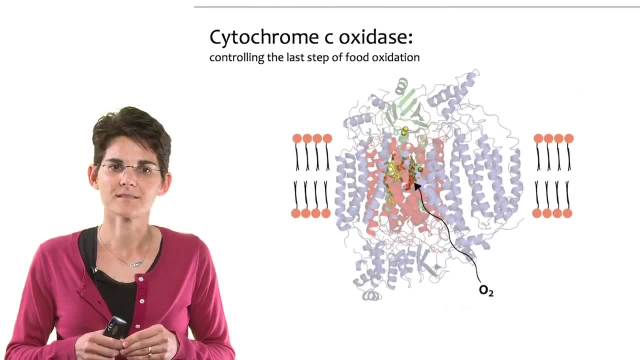 here's a protein called cytochrome C oxidase. it's a membrane protein. that's what those squiggly lines are on the side with the orange dots. that's the lipid membrane of your mitochondrion and that big protein is cytochrome C. 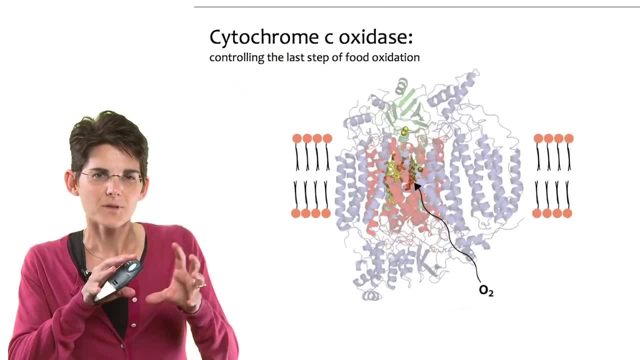 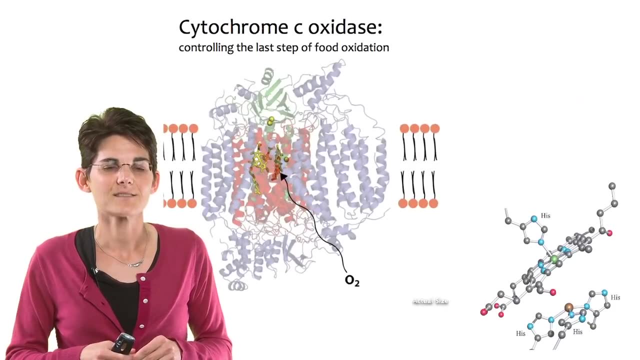 oxidase. and if you zoom in it to the center of your mitochondrion and you zoom in it to the center of your mitochondrion and you'll see a couple other things in there. you'll see the o2. you can see where that goes into the middle of the protein. and if we look into that active site, you 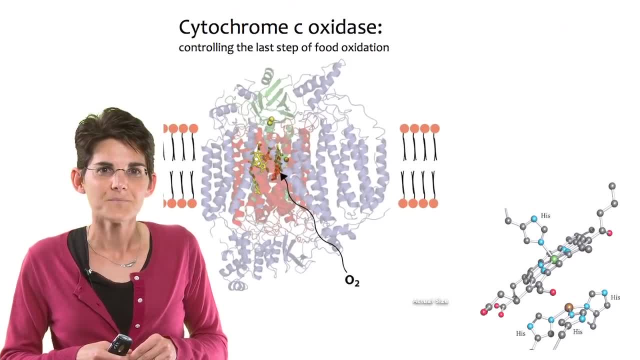 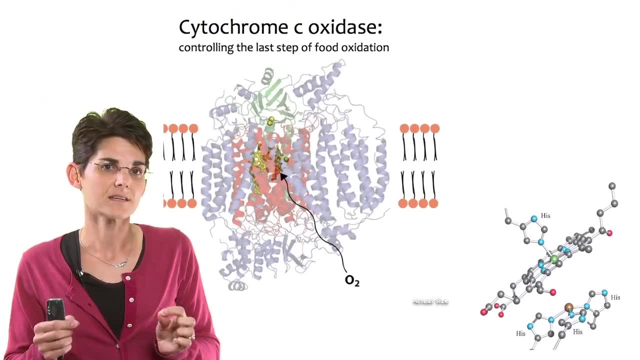 see more inorganic chemistry. so here's an iron porphyrin. the iron is the green dot in the middle of the porphyrin ring and underneath that is a copper surrounded by six nitrogen donor atoms on histidines. those are amino acid side. 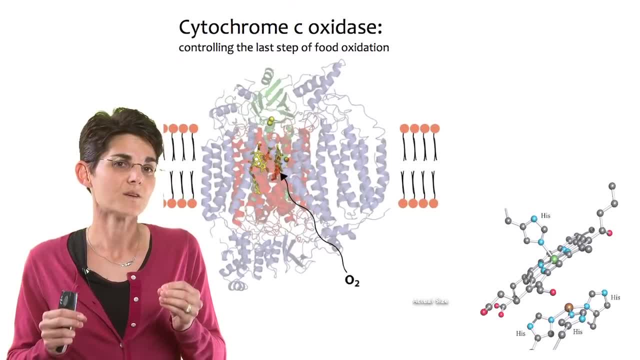 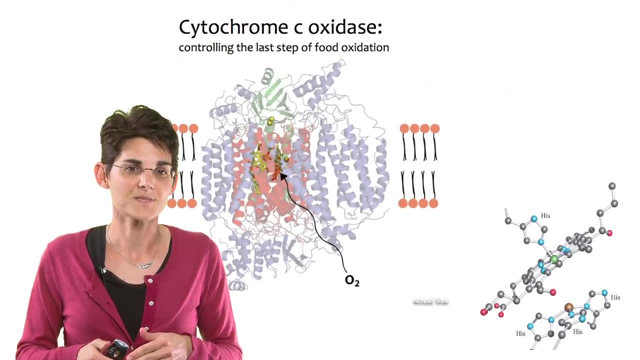 chains on the protein and oxygen is going to bind in between those two metal centers and ultimately turn into water. there's another inorganic site, another metal cofactor, that's on cytochrome C oxidase and that's up here, a two copper center. so this brown, bronze colored or 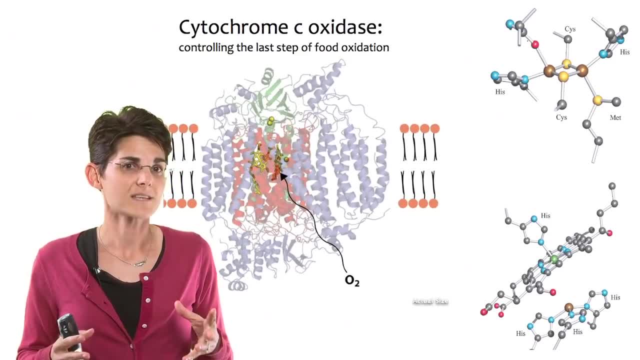 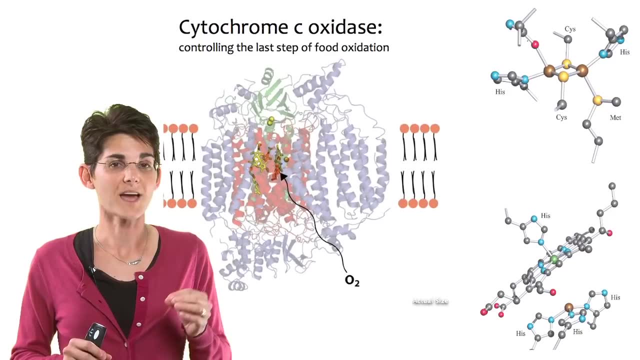 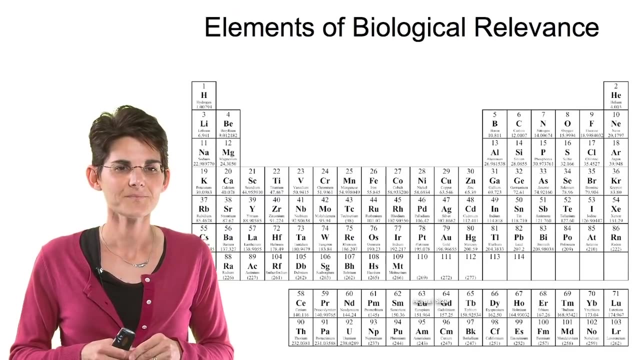 copper colored spheres are the two coppers and again it has amino acid side chains that hold that copper center into place. so here's just two small examples of metallic cofactors found in a protein that's involved in an essential life process. that's not organic, but it is living. so now that we've looked at the 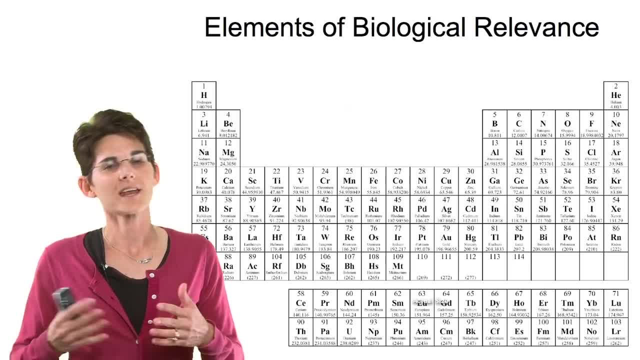 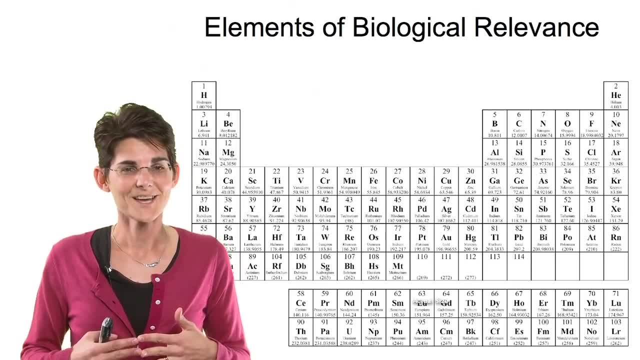 now let's take a look at the rest of the periodic table. we said that organic chemistry was carbon-based and inorganic chemistry is non carbon-based. we have a lot of elements to deal with in inorganic chemistry. so here's our periodic table of the elements, and we'll start with the bulk biological elements. 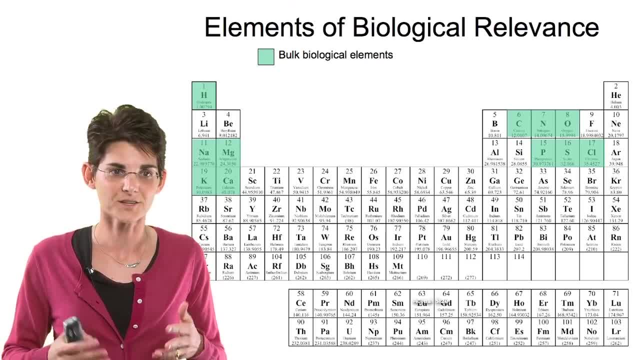 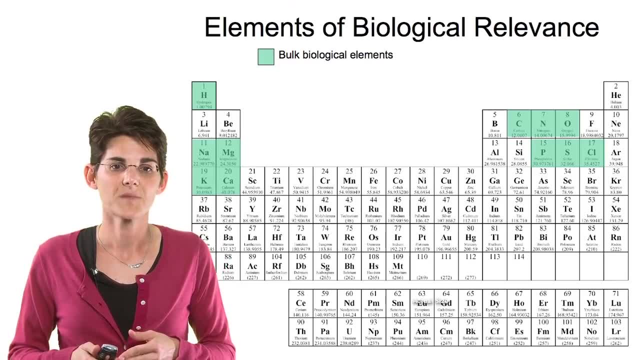 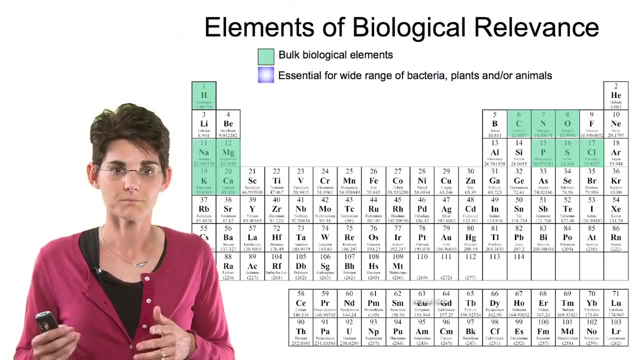 these are the things like carbon, hydrogen, oxygen, sulfur, then the metal ions like sodium, magnesium, potassium and calcium, of course, hydrogen. so those are the bulk metals, or bulk elements. now we'll look at the elements that are essential for a wide range of bacteria, plants, you and me, and you'll see that we go mostly across the whole first row of 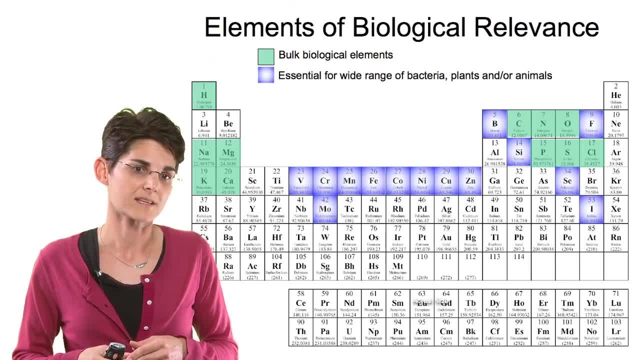 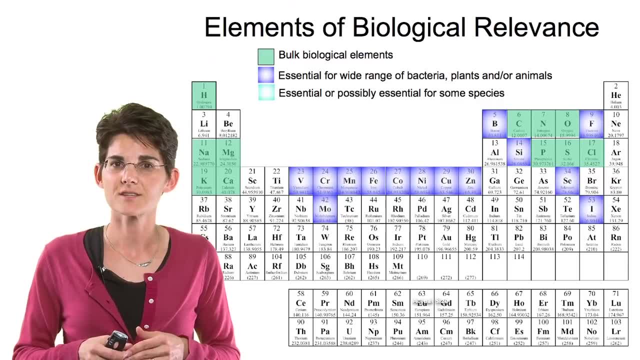 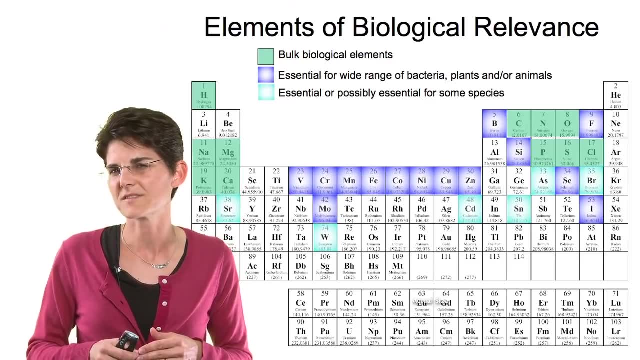 the transition elements and we have a lot of the rest of the p block that gets filled in, but notice, not all of the people. so then we have elements that are essential or may be essential for some species, but not necessarily all, and you'll notice on this list we have a couple. some of these are still somewhat 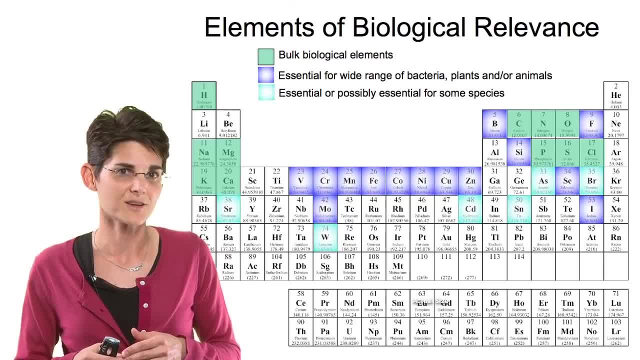 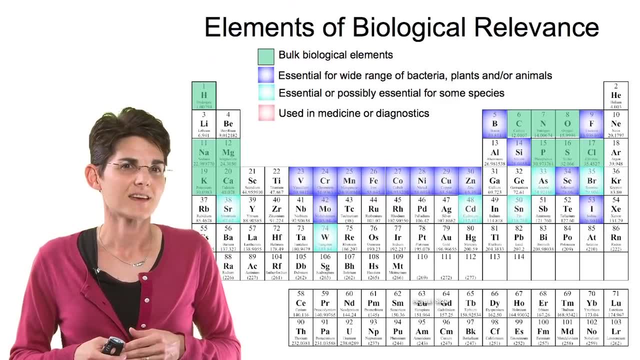 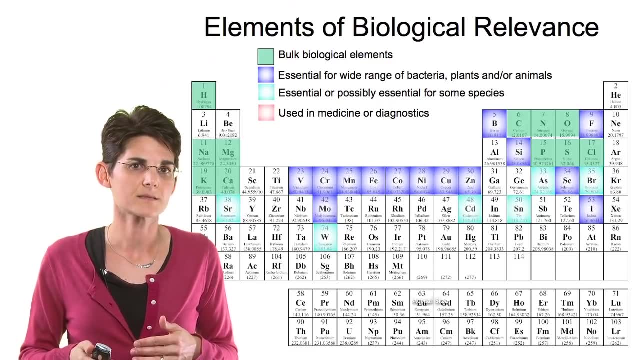 controversial. They might be essential for some strange bacteria that live in ocean vents, but they might not be essential for all organisms. And then we have another set that inorganic chemists also play with, and these are elements that can be used in medicine or diagnostics, but they're not necessarily naturally occurring. 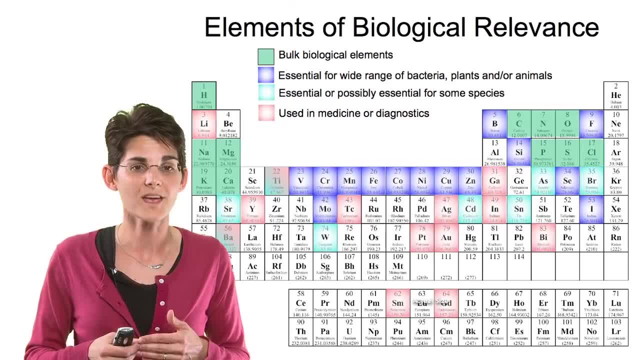 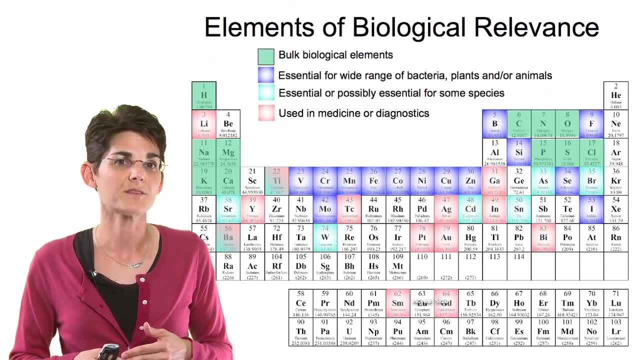 And here we have a list that's growing. so chemists can be quite creative, and a lot of these elements have different kinds of properties and people take advantage of those to do a lot of different things. So here are just a couple of the examples. 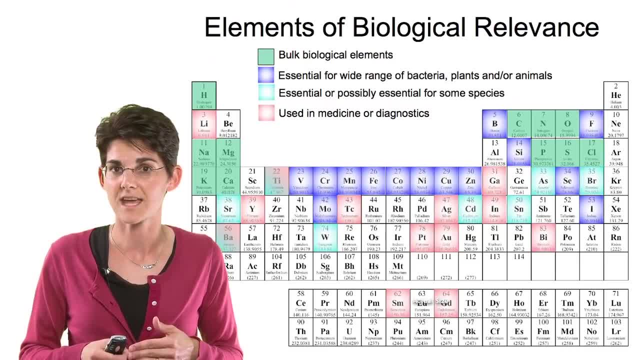 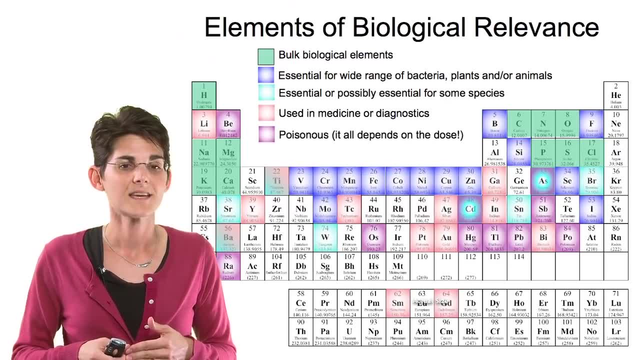 One famous example is platinum. that's used in a widely used anti-cancer agent, cisplatin, But there are a lot of others and there are more on their way. And then of course there are ones that are poisonous, And here again I haven't covered in everything. but the poison all depends on the dose. 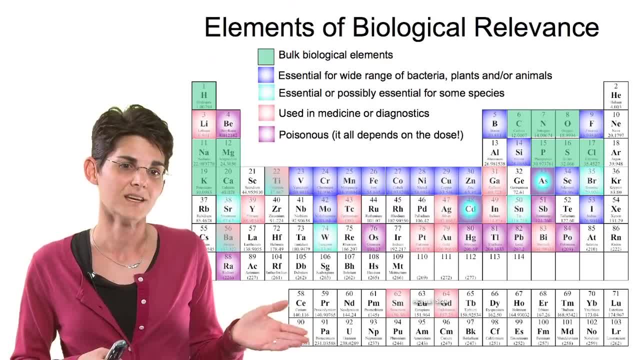 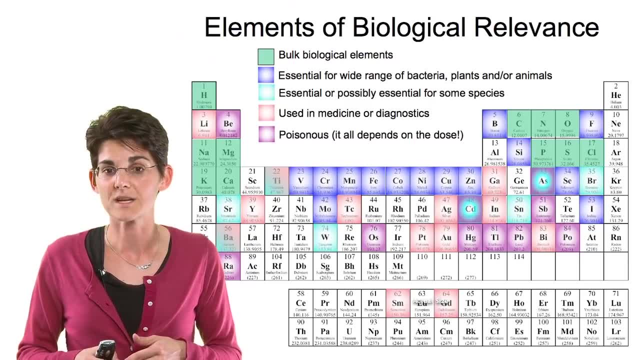 So really most of these elements can be toxic at some concentration. but some of the other toxicities you'll recognize- things like mercury or thallium or lead- we know are inherently pretty toxic And we don't have an essential ingredient. 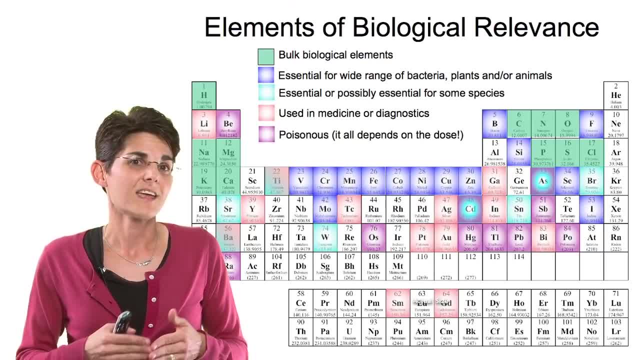 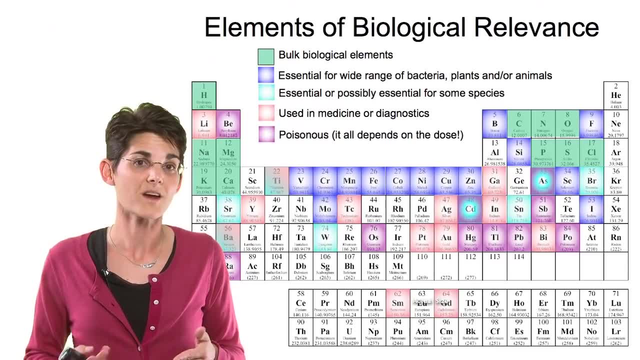 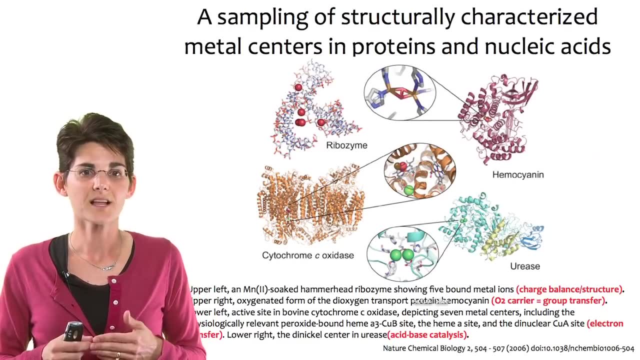 We don't have an essential function for those elements. So you can see that inorganic chemistry has a lot to do with life and living things, And inorganic chemists who do biological inorganic chemistry have the whole periodic table to cover. Here again we'll look at just a couple of examples of metalloenzymes or metallobiomolecules. 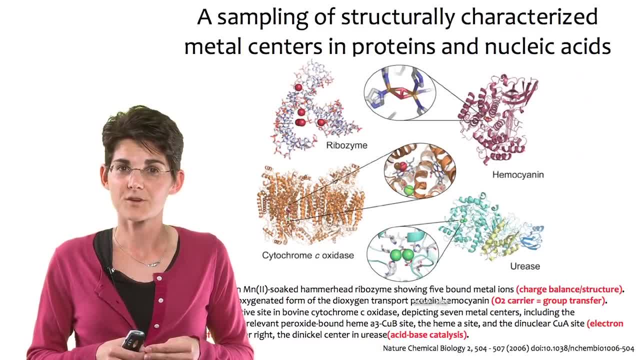 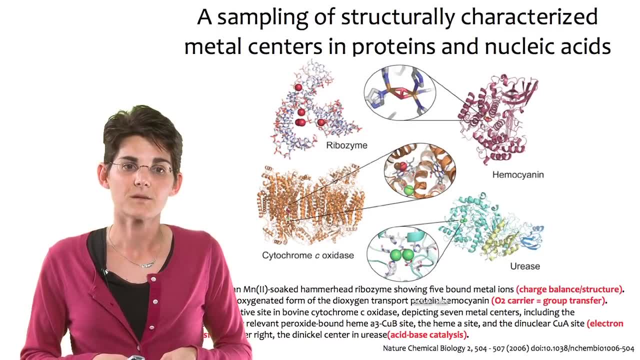 that have metal cofactors. We already talked about cytochrome C oxidase and the iron and copper that's found at the active site of that molecule, But also on this list there's the ribozyme, and that has metals that can hold it into. 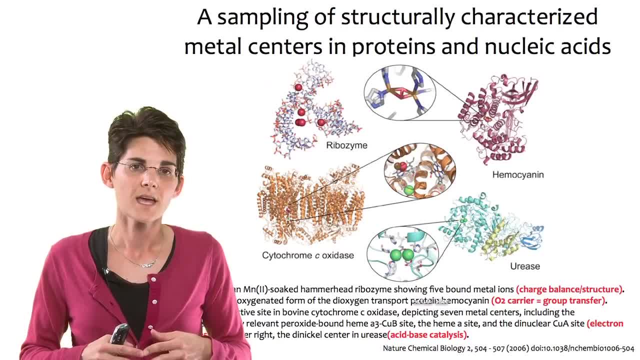 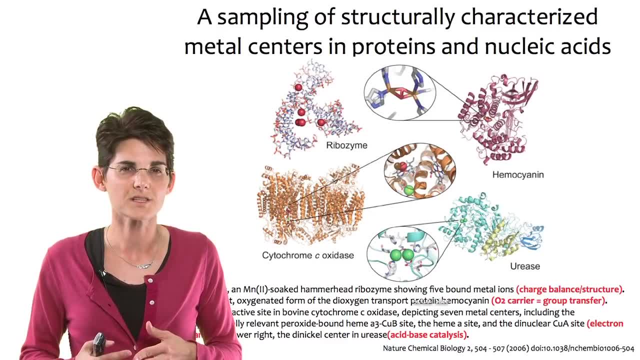 place. So there's an example of nucleic acids with metal cofactors. You can see that the purpose of the metal ions there is to hold some charge, balance and maintain structure. So that's one of the functions of metals that can be used in biological chemistry. 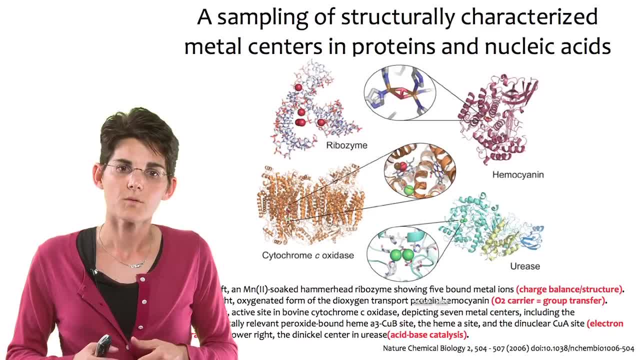 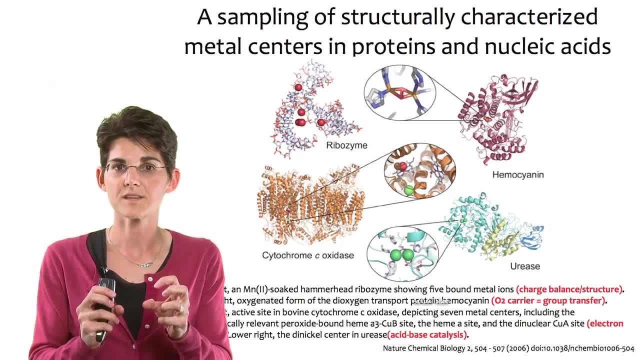 Also on this list or on this just small example, we see urease. Urease is a nickel enzyme And you'll see that in the structure there are two green spheres. Those are the two nickel atoms. Urease is one of the first enzymes that was solved by X-ray crystallography. 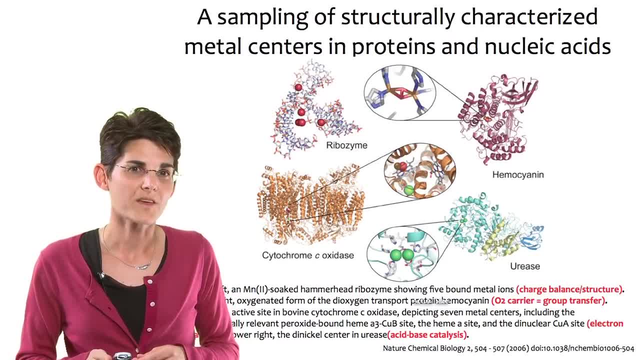 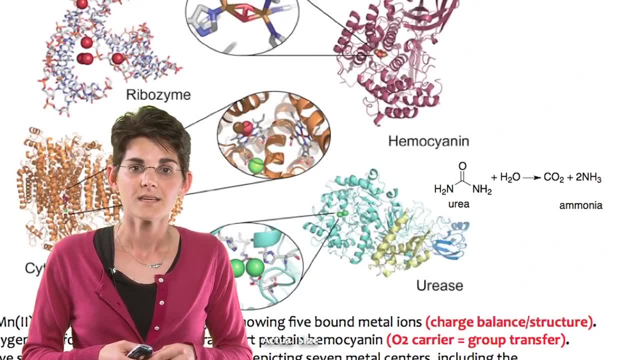 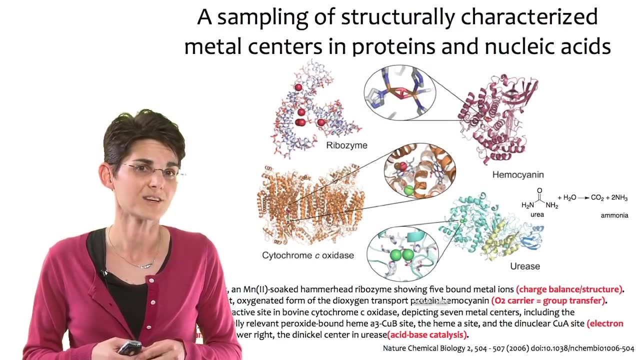 And that's where they discovered the two nickel sites. If you want to know what the chemical reaction is that urease does, here it is. It hydrolyzes urea to give CO2 and ammonia, And this is an enzyme that's not found in humans, but it is found in some bacteria. 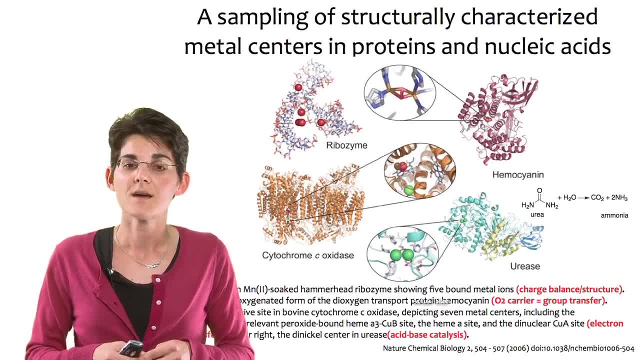 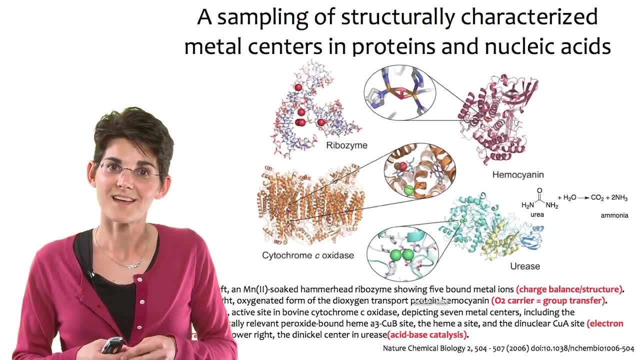 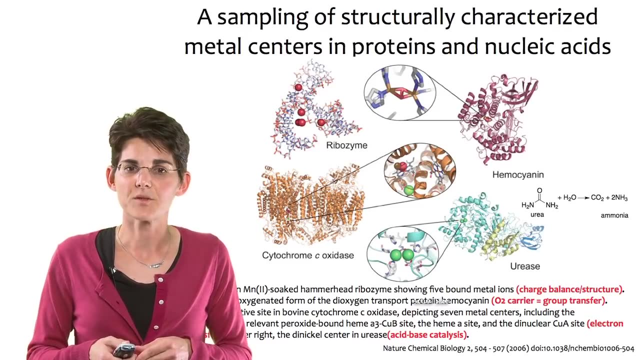 bacteria that live in your gut- so these are the helobacter pylori. bacteria that causes ulcers- has to live in an acidic environment, but if it has a lot of urease it forms a lot of ammonia and that acts to stabilize and buffer their system so that they can survive in an acidic environment. and the last example: 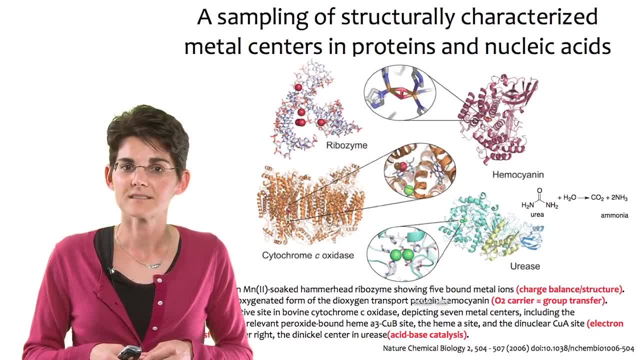 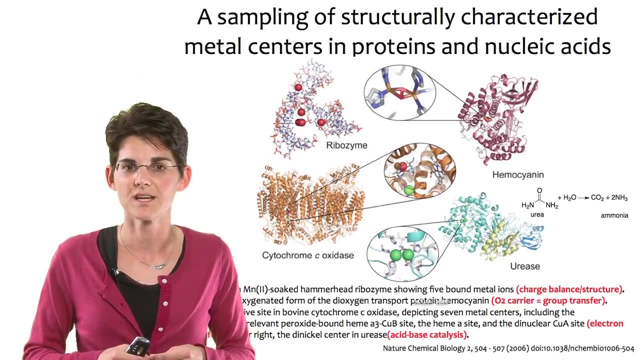 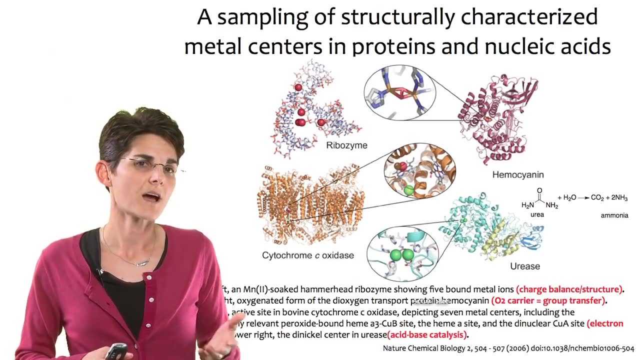 that we'll look at a little bit is up at the top and that's hemocyanin, and you'll see there are two yellow, brown connections. those are really the copper atoms that are drawn in that structure. so here's a copper containing enzyme. again, this one's found in arthropods and it carries oxygen. so you and I, we use 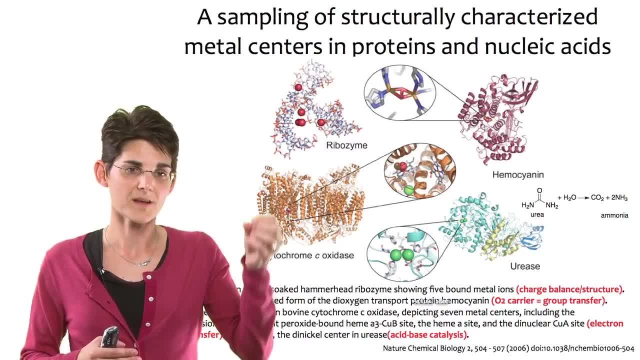 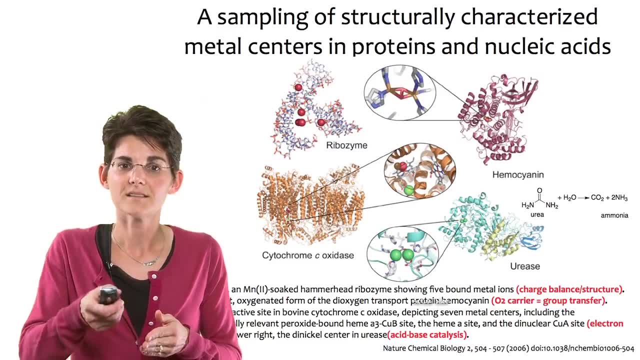 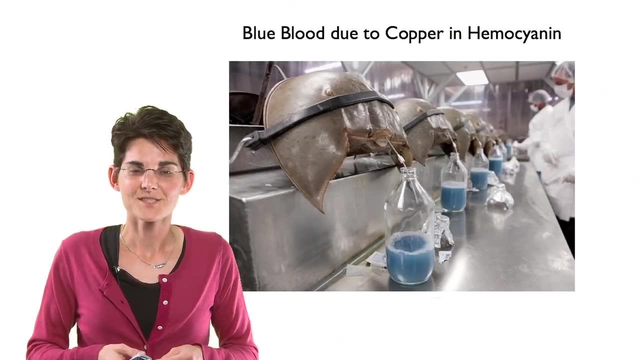 hemoglobin to carry our oxygen. that's actually an iron center that binds oxygen. here hemocyanin- and arthropods- uses copper and it binds oxygen in between. so you see the red line that's between those two coppers, that's the o2 that's coordinated to hemocyanin. so what are arthropods? so here's one example and 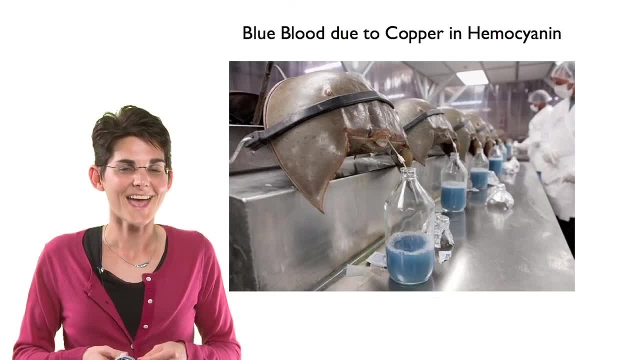 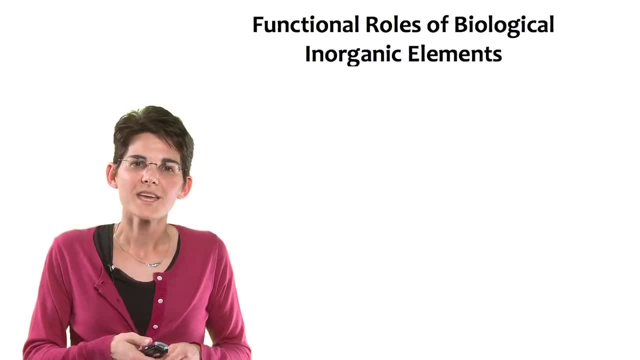 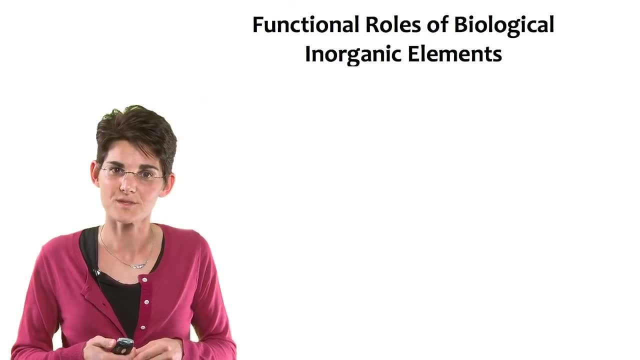 two coppers. that binds oxygen and gives a really nice blue color. so now we can summarize many of the functional roles for for one, of the biological roles for inorganic elements that are used in biology. we haven't looked at all of these, but hopefully you'll get a little bit of an appetite to start looking for. 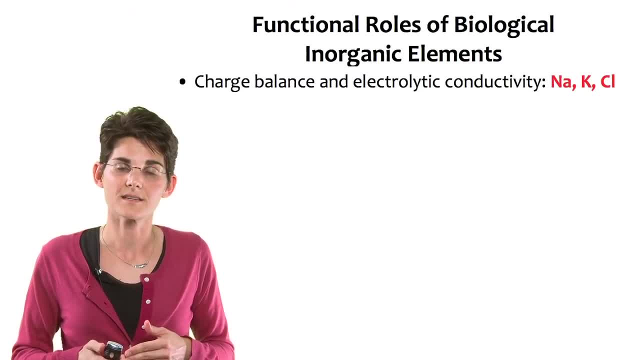 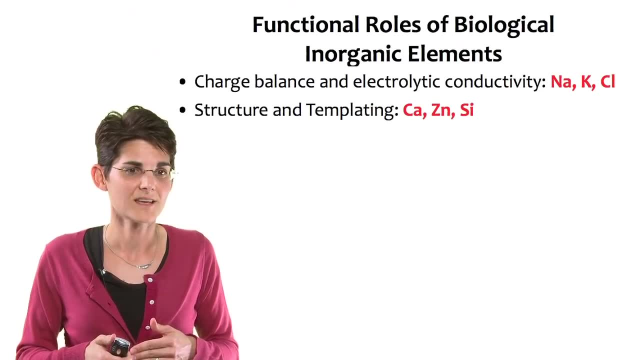 more so. one are simple things like charge balance and electrolytic conductivity, structure and templating things that hold other things together. think about your bones, made of calcium and phosphate. that's one example, but you can also see the smaller examples in proteins where a metal cofactor could help with with a. 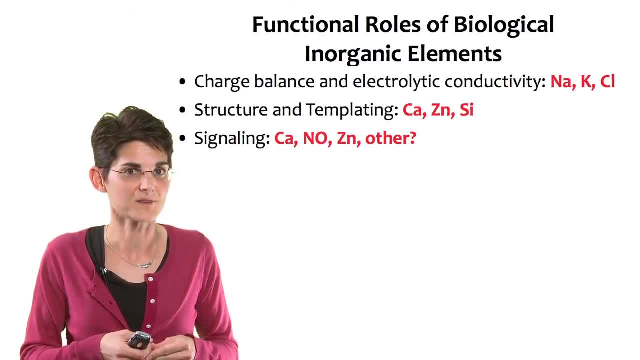 structural feature, signaling molecules. so these are molecules that- calcium or no- that have to come on and off and cause some biological signal in inside a cell or between cells. and then there are things that you'll be hearing a lot about in general: chemistry: Bronsted, acid-base, buffering or Lewis acid-base.